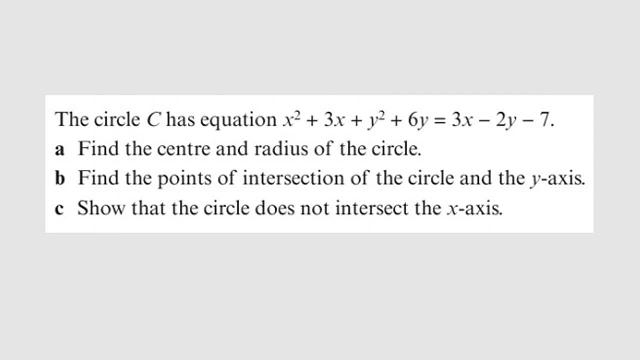 Hello, good day viewers. Still on coordinate geometry, here is our problem for today. The cycle C has an equation, x squared plus 3x plus y squared plus 6y, equal to 3x minus 2y minus 7.. We are asked to find the centre and radius of that cycle. We are asked to 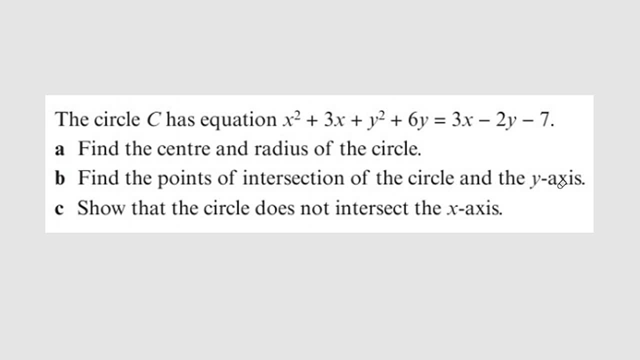 find the point of intersection of the cycle and y axis, that is, y intercept, And also we are asked to show that the cycle does not intersect x axis. Alright, let's get started. I think for the first question I am going to show you two different ways to do that. 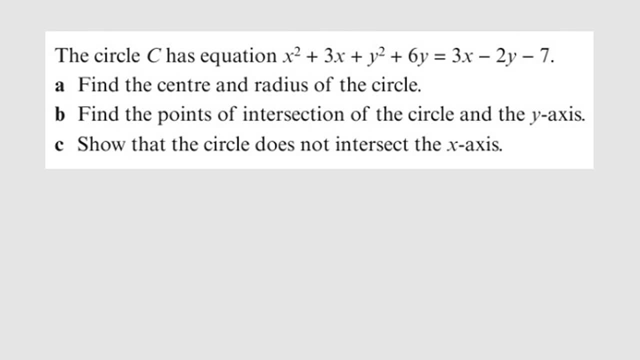 We are going to use the general form and the standard form. The equation we are given is x squared plus 3x plus y squared plus 6y. This is equal to 3x plus 3y minus 7.. We are asked to find out the partial angle minus 2y minus 7.. Let us bring every term to the 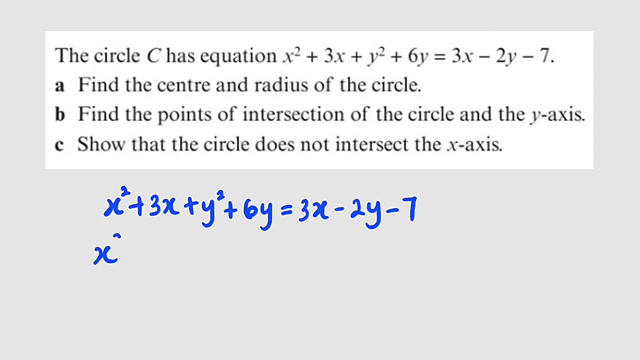 left hand side. We have x squared. here We have plus 3x. If this crosses over, it becomes negative 3x. Then we have y squared, We have 6y. If this crosses over, it becomes positive, We have plus 2y. 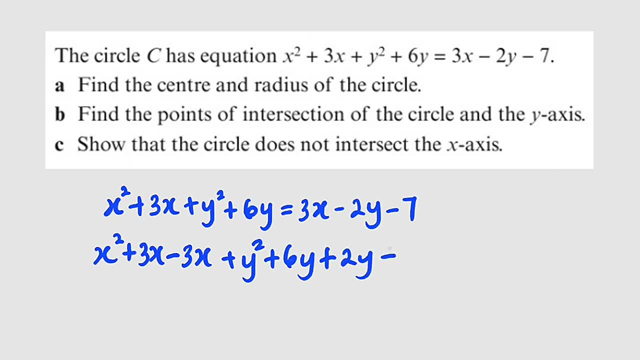 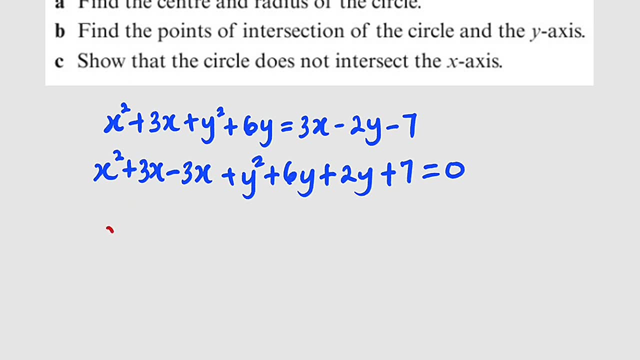 We have x squared, We have 1x. If this crosses over, it becomes positive as well, and the whole of this equals 0.. Now let us simplify this. We have x squared plus 0x, for a reason, plus y squared plus 8y, then plus 7.. 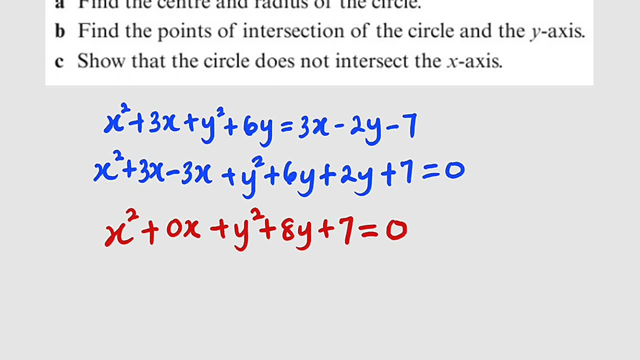 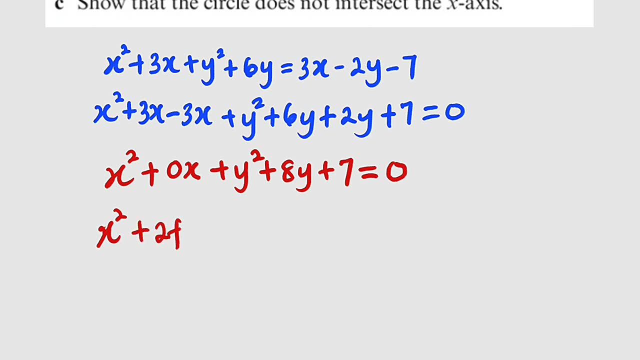 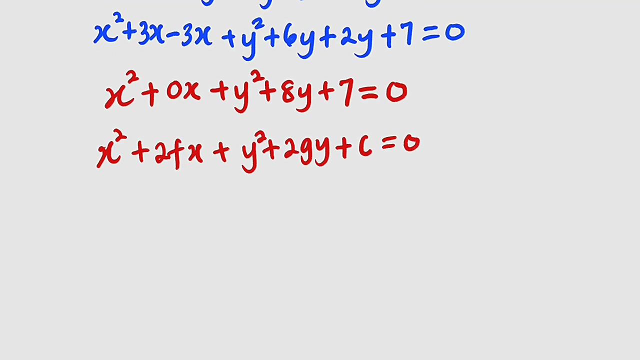 The whole of this equals 0.. This equation is in general form, which we can write as: what x squared plus 2fx, plus y squared plus 2gy, then plus c, The whole of this equals 0.. Where the center of that cycle is given us, let me write it here: center. 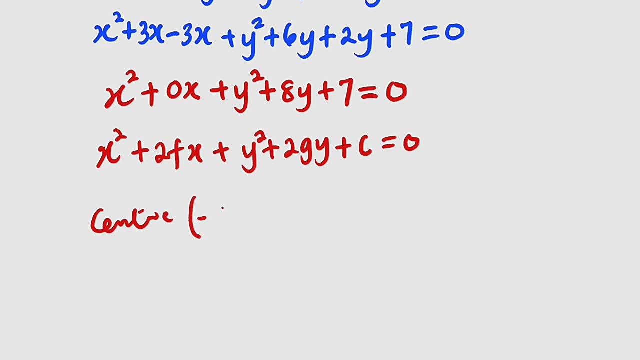 The center has the coordinates negative f, negative g, And the radius can be obtained by taking the square root of f squared plus g squared minus c. This is our value of c, which corresponds to 7 here. Alright, let us find these values. 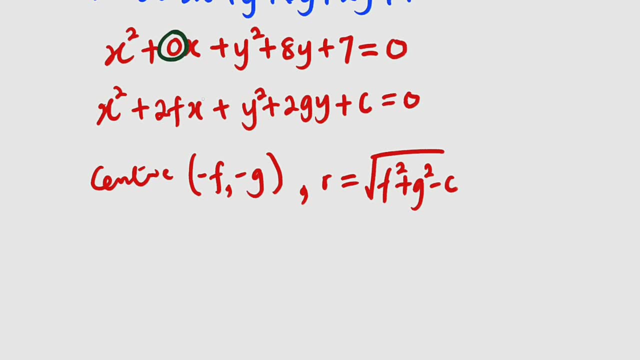 If we start with f, you can see the coefficient of x here is 0,, while the coefficient of x here is 2f. So it means that 2f is equal to 0, which means that f also equals 0.. 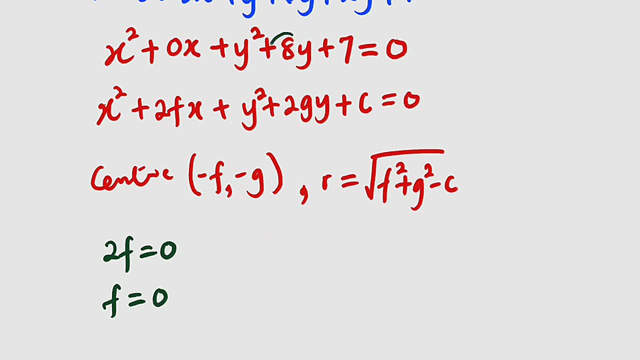 It must be equal to 0. And the coefficient of y is 8 here, while the coefficient of y here is 2g. So we have 2g equal to 8.. And if you divide both sides by 2, you have g to be equal to 4.. 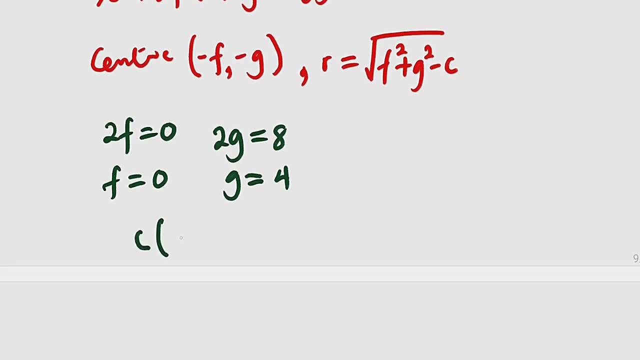 So what will be the center? The center of that cycle will be negative f, f is 0,, negative 0 is still 0, then comma negative g, g is 4, and negative of that will be negative 4.. 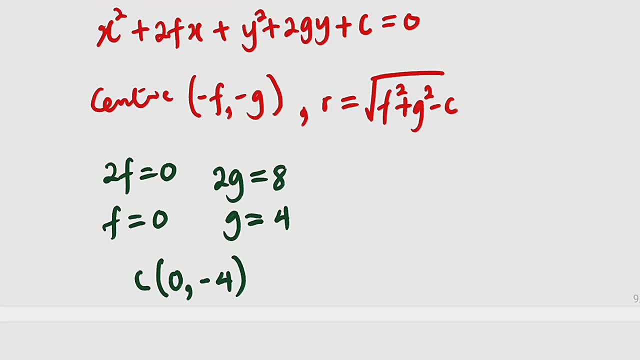 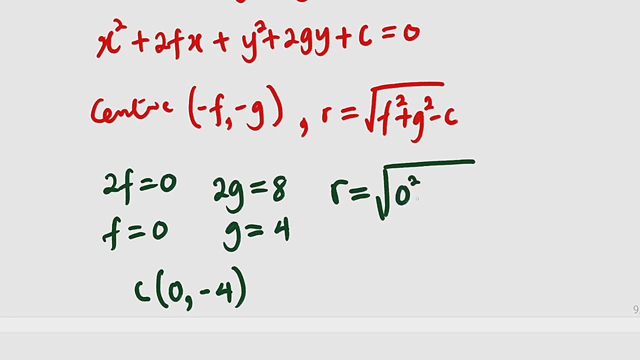 And hence this is the center of that cycle. So what about radius? To find the radius r, this is equal to the square root of f squared, that is, 0 squared, plus g squared, which is 4 squared then minus c. 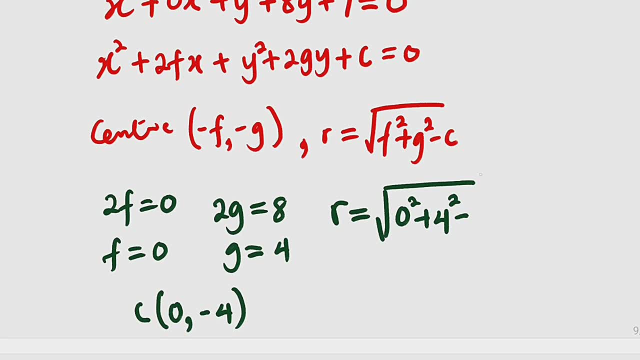 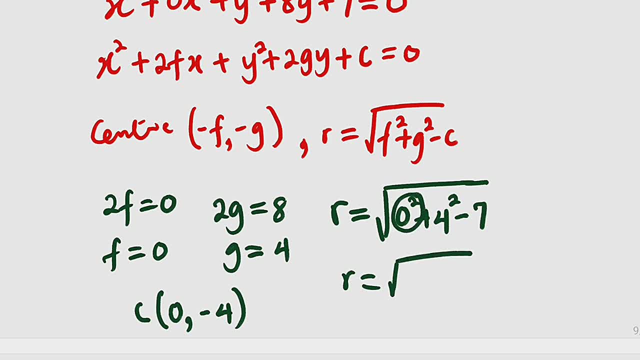 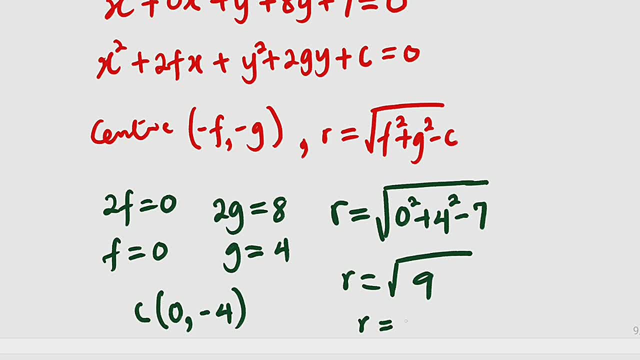 So this is square root of 9.. And square root of 9 is equal to 3.. Remember, r is radius, which is a distance, So we should expect a positive result. So this is all about a part, And I promised to show you two different ways to do that right. 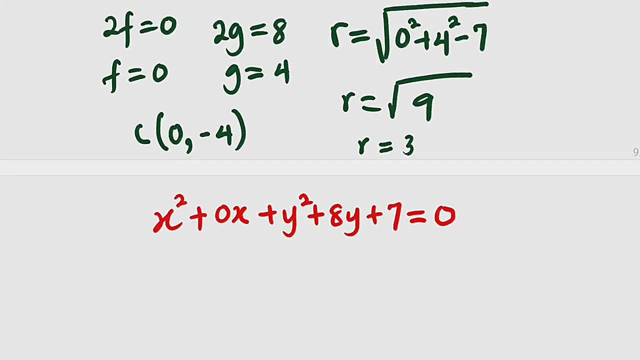 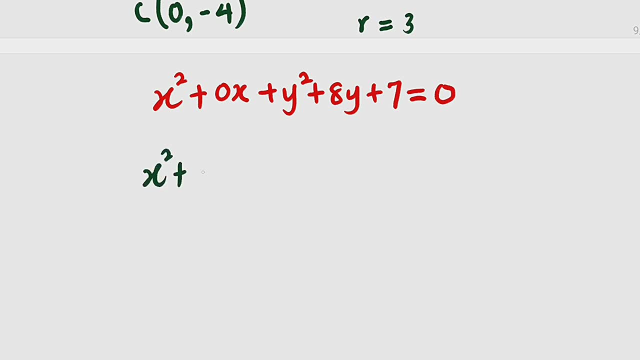 So I would like to copy this equation. This is the equation I would like to translate, transform into standard form. so this is x squared plus zero x. to make it a complete squared you have to take the square of half of the coefficient of x. the coefficient of x is zero. half of that is still. 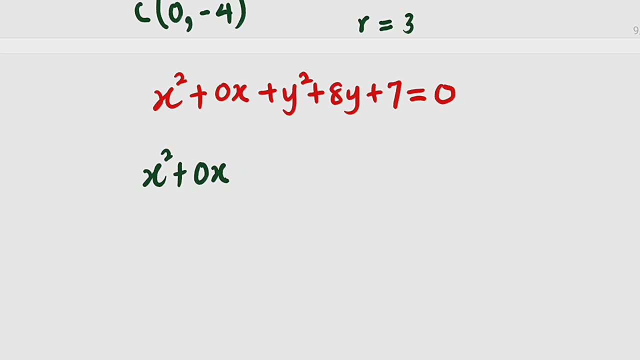 zero squared is also zero, so it's like we are adding zero here, which we don't have to. then plus y, squared, plus eight y, to make this a complete squared. you take half of this, which is four, you square that, you get 16, right, remember we are taking seven to the other side. it becomes negative. 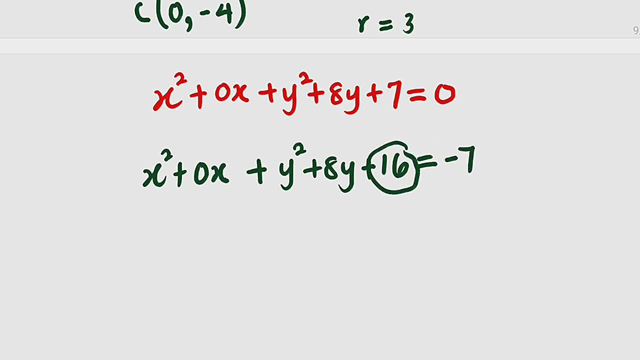 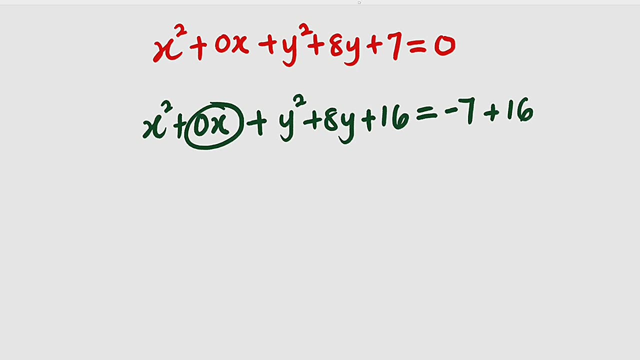 seven. and since we have added 16 to the left hand side, we have to add it to the right hand side to make the equation balance right. so you know, zero x is still zero. so we have x squared here plus. if you want to factorize this, you take y, then half of this is 4. we have 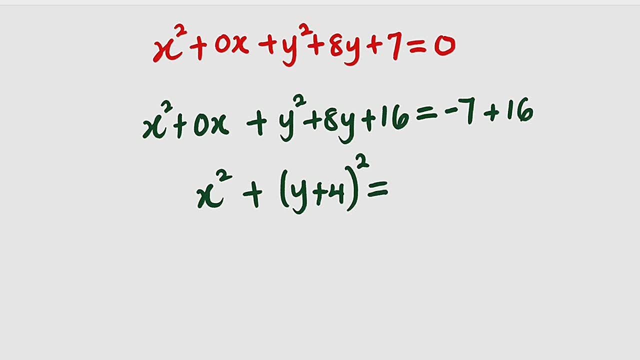 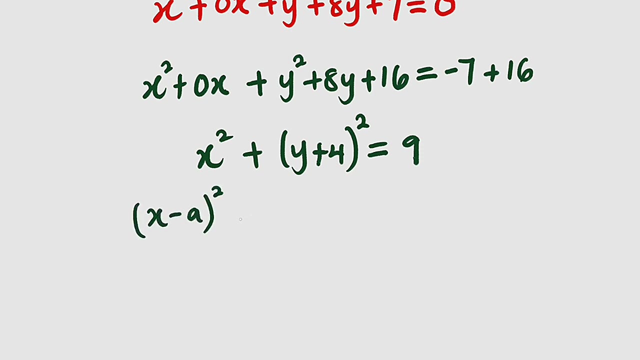 plus 4 whole squared, and this is equal to negative. 7 plus 16 will give us 9, so this is 9. so this is our equation in standard form which, if you can remember, we can write as: X minus a whole squared, plus Y minus B whole squared equal to R squared, where we say that the center of that cycle will be what? 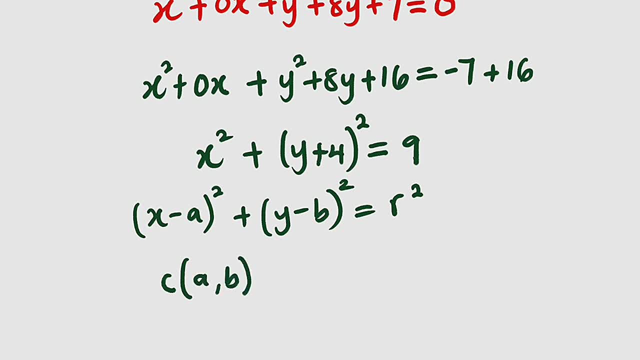 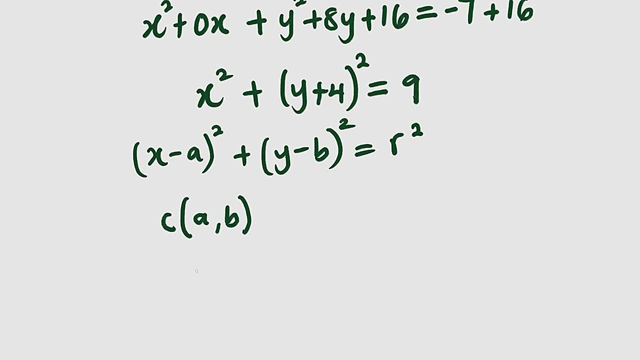 a, comma B. so now let us start with the center a here. you can see we have no a here, so we are going to consider it as 0. so the center x coordinate is 0, then B is this value here, that is negative 4. we have. 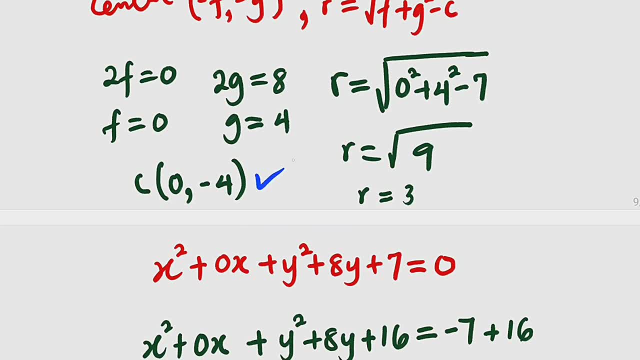 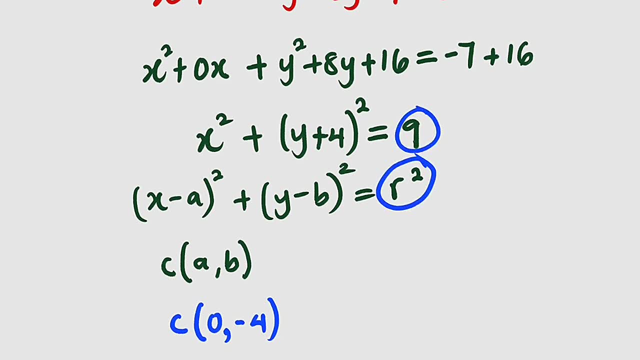 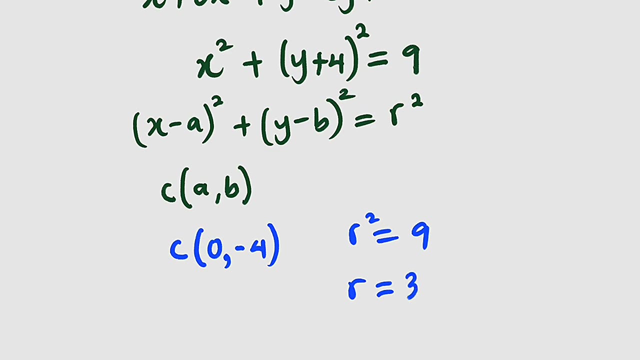 negative 4. you can see they're exactly the same with the previous one, 0 comma, negative 4 and the right hand side. you can see that R squared will be equal to what? 9. so R squared equal to 9, which implies that R must be equal to 30. you see, the radius is equal to 30. so this is all about the. 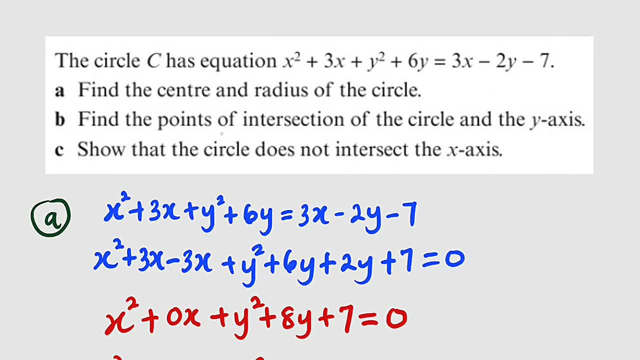 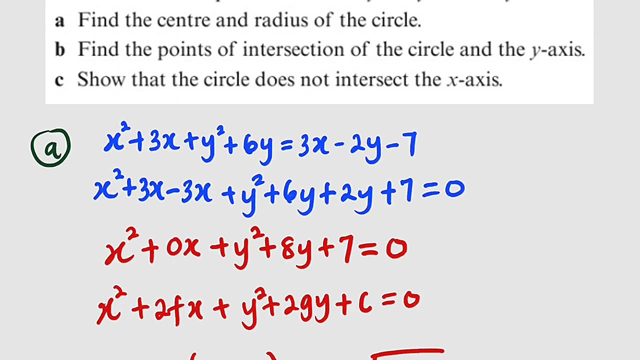 first question. then, going to the second question, we are asked to find the points of intersection that are in that circle Y, and that is exactly where the circle crosses Y axis, and it can be of 10, by setting the value of X equal to 0. we can take either of these equations either in standard. 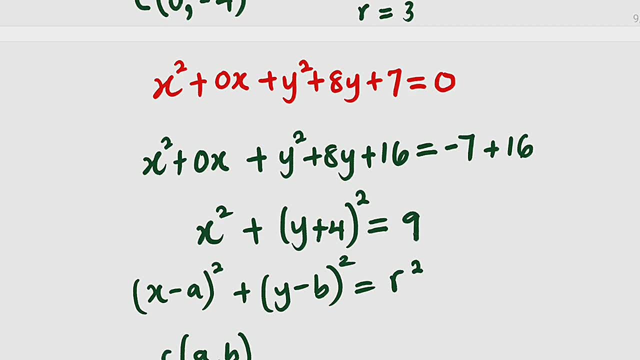 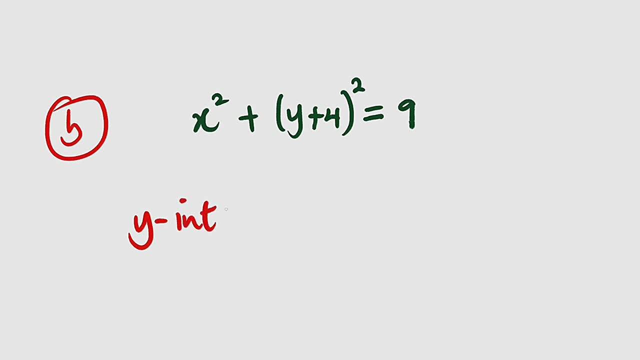 form or in general form, it doesn't matter. so I think let me take the equation in standard form. so B part, we are looking for Y intercepts. that's exactly where X is equal to 0 and then we are to 0. so if we set X to be equal to 0, the whole of this will be 0, right? we only 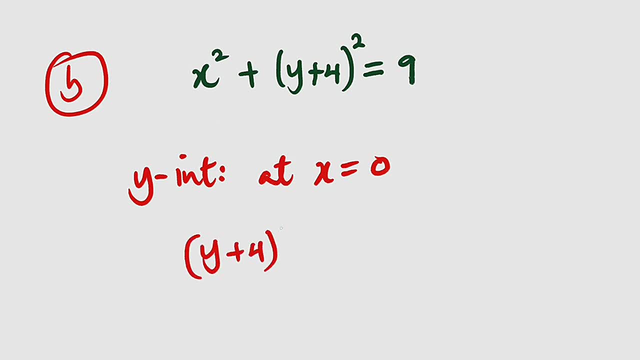 have y plus 4, whole squared equal to 9. let's take square root of both sides. we have y plus 4 equal to plus or minus. the square root of 9, y plus 4, is equal to plus or minus 3. therefore, Y will be equal to minus 4 if you take this to the 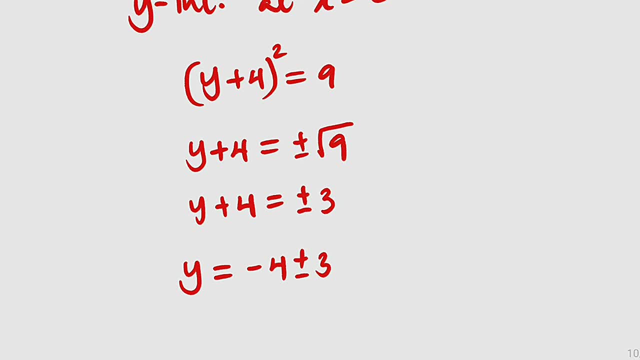 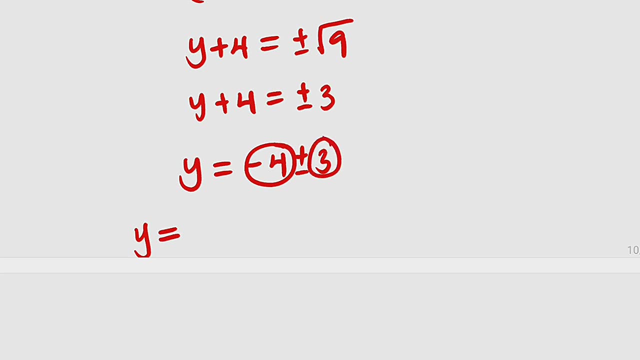 other side plus or minus 3, meaning we have two values of Y. Y could be negative, 4 plus 3, which is going to give us what negative 1. so we have negative 1 or negative 4, negative 3, which is negative 7. 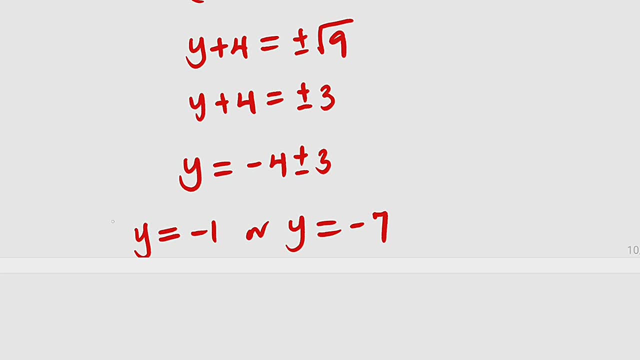 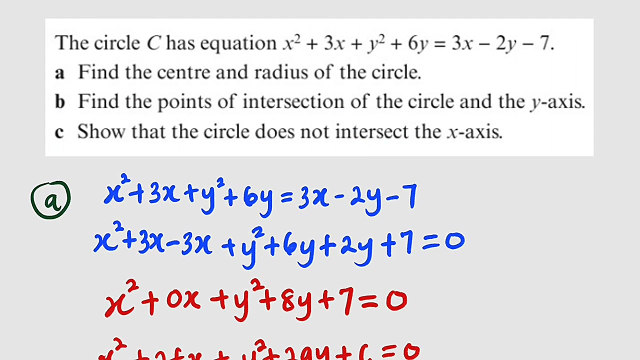 so this is negative 7. so these are exactly the points where the cycle crosses Y axis, all at the negative side. then the last question: here we are asked to show that the cycle does not intersect X axis, meaning there is no X intercept. you know, X intercept is the value of X when Y is equal to 0. so now let us pretend as if. 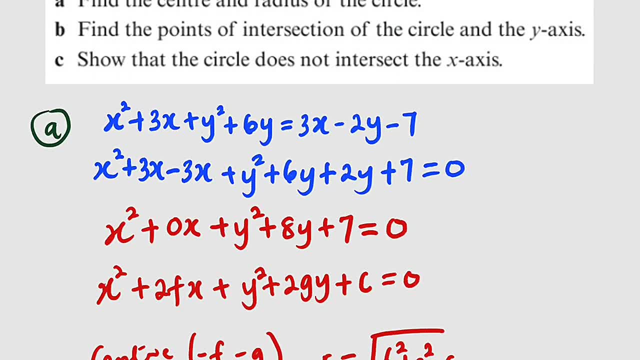 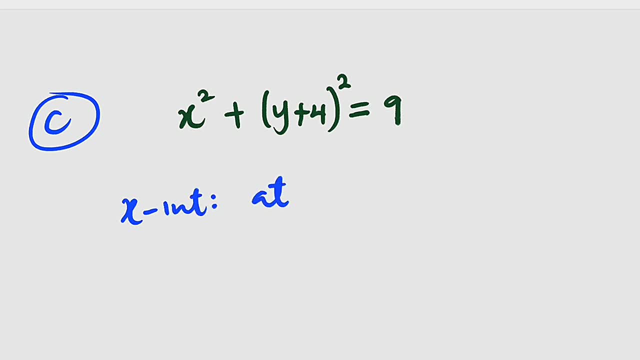 we have X intercept by setting Y to be equal to 0. so this is the C part. we are looking for X intercept letters at Y equal to 0, which means what X squared plus 0 plus 4, because 1 is 0, this is: